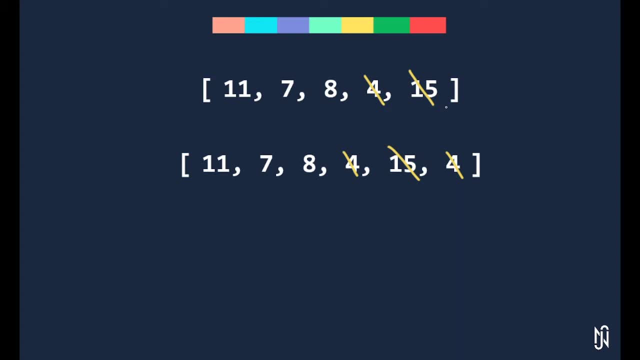 So how are we going to go about solving this? So the first thing we want to do is figure out what the smallest number is and what the largest number is, And we can do that by setting variables for the lowest and for the highest. We can use the. 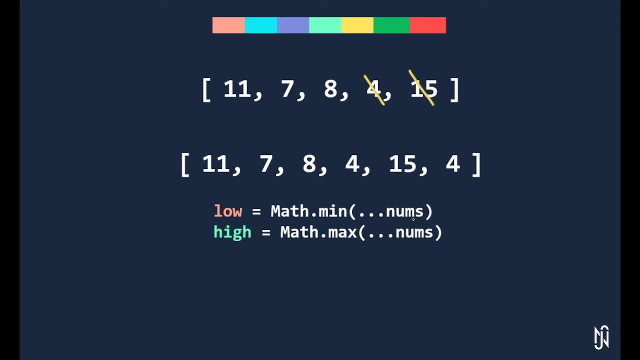 Spread operator to spread the nums array and then use the math dot min function to find the smallest number, and then then we'll set that to low. And again we'll spread the nums, use the math dot max function and we'll set that to high. So now we 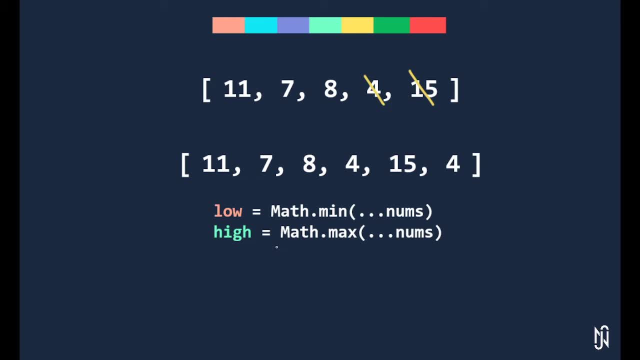 have our lowest number set to a variable and our highest number set to a variable, And so to get the number of element elements in this array that are not equal to low or high, what we can do is we can create a counter. so we'll just create count over here. 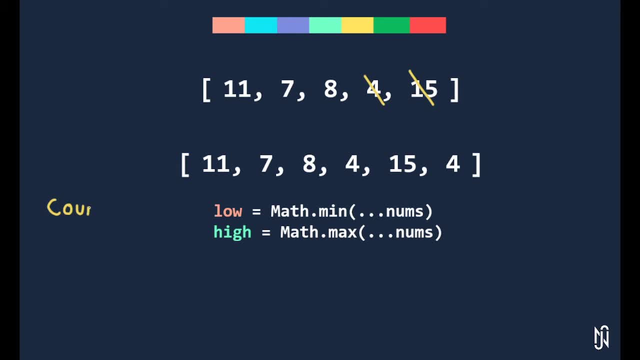 and what we're going to do is we're going to loop through the array and we're going to check to see whether or not the current index number is not equal to low and not equal to high. so we can use a conditional as we loop through: if num's i does not equal low. 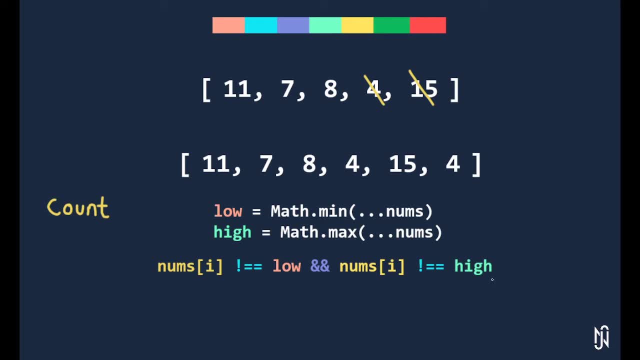 and num's. i does not equal high. we're going to add to our count. so let's run through this first example: uh, 11. or we're going to set low and mathmin will return 4, and then we're going to look for high, which is 15, so we're going to set that. 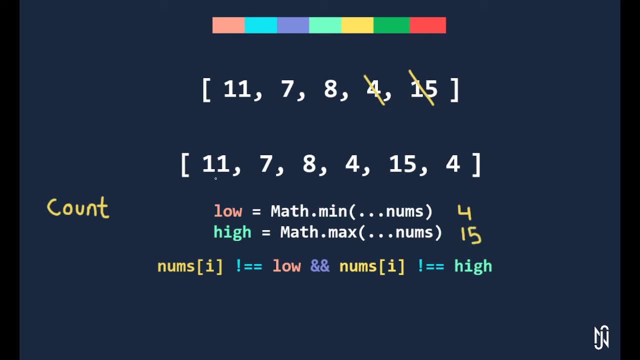 and then, as we loop through the array, 11 does not equal 4 or 15, 7 does not equal 4 or 15, 8 does not equal 4 or 15. so now we're at 3 for our count. 4 does equal 4 or 15, 15 does. 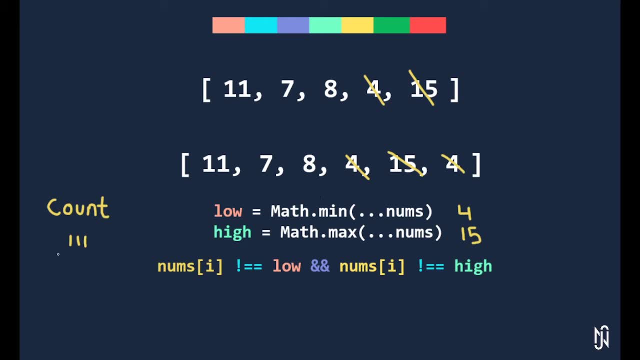 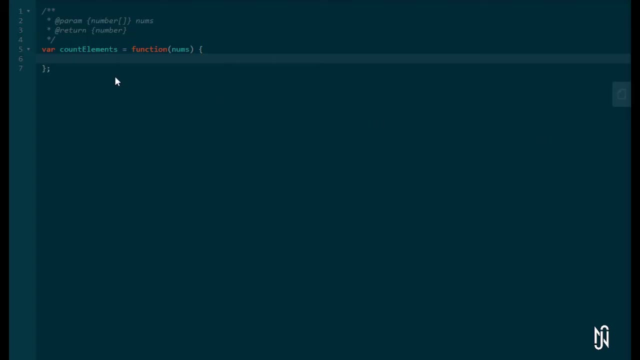 as well, and so does 4.. so that will give us the answer 3 that we are looking for. so that does it for our diagram. let's try typing this in code. so we want to start out by setting our low and our high variables as we diagram that out. 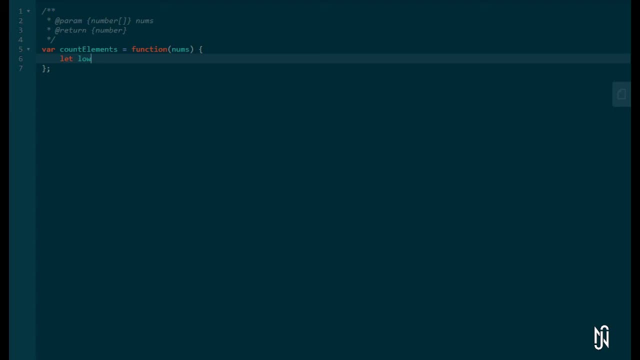 we want to use the math dot min and mathmax functions, so we have let low equal math dot min. we're going to use the spread operator on the nums array. then we want to get our highest number, so we'll set that to high equals math dot max on nums as we spread it. and we also want to 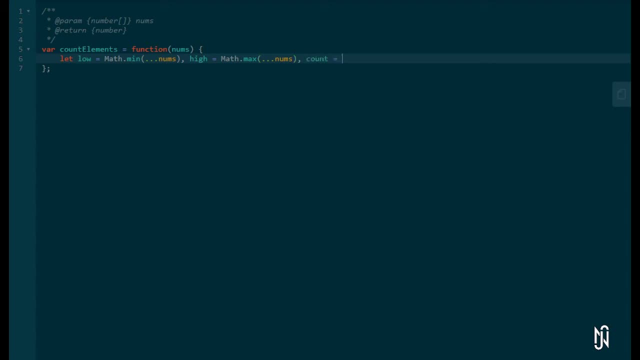 substantiate our count. so we'll set count equal to zero and at the end we want to return our count as our answer. so we're going to start our for loop. we're going to set i equal to zero. i is going to be less than nums dot length. 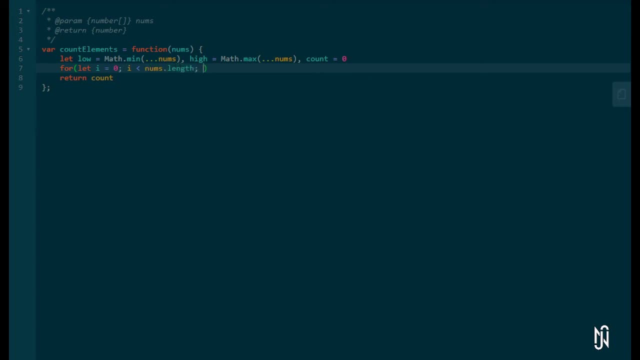 and we're going to increment i at every pass. now we're going to want to use our conditional that we used in the diagram to check whether or not the current iteration of nums is equal or, in this case, not equal to low and not equal to high. 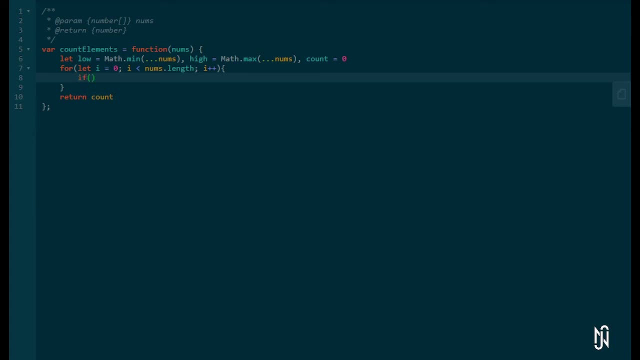 so we're going to say if nums i does not equal low and nums i does not equal high, we're going to want to increase count by one. and that's it for this code. i am going to run this with the test cases and see if there's any mistakes. 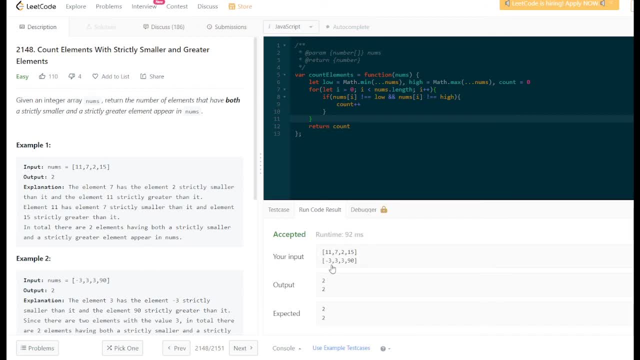 and it comes back as accepted. so this is pretty good. um, we don't have to use the test cases for this code. so we're going to run this with the test cases and we can add more cores if we use them. and here's a good example of what the check result is. 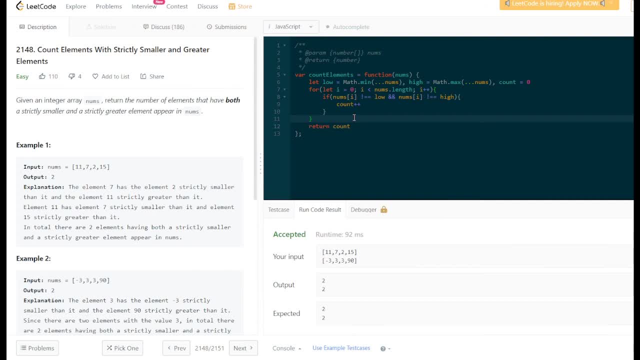 so what i believe is that we don't need to use a loop and, in fact, we don't even have to use a count. we can refactor this into a more streamlined solution using the filter method on the nums array. so what i want to do is remove this loop and then remove this count.